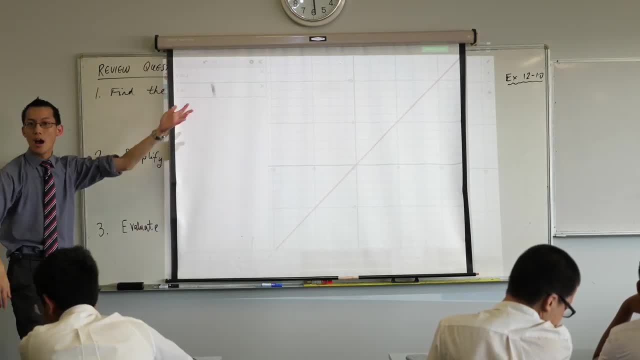 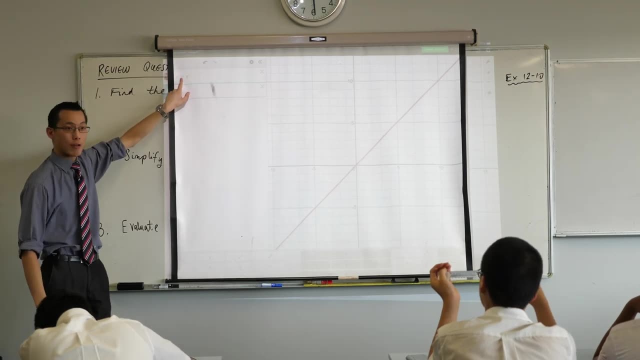 is these straight lines that we're getting from. these equations are going to cross paths with each other. they're going to intersect. Okay, now you can see. I have already- and I invite you to do the same, I've already graphed the first equation in the first question 1a: y equals x. and then you can see. 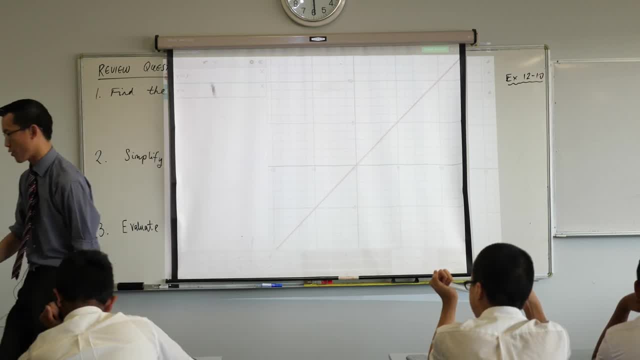 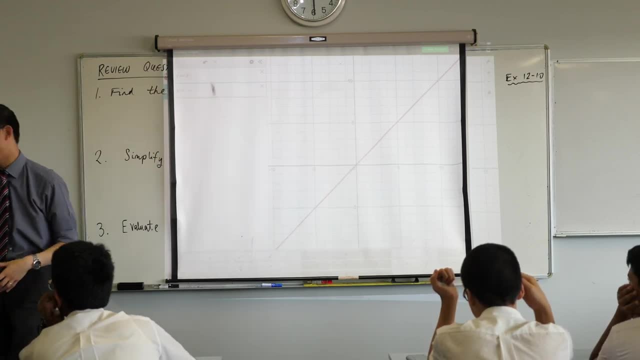 they provide you with a second equation which will give us a second straight line. So go over into Desmos and you can see. if you hit enter, you can put a new line in there and you'll see both at the same time. The second one has an equation. 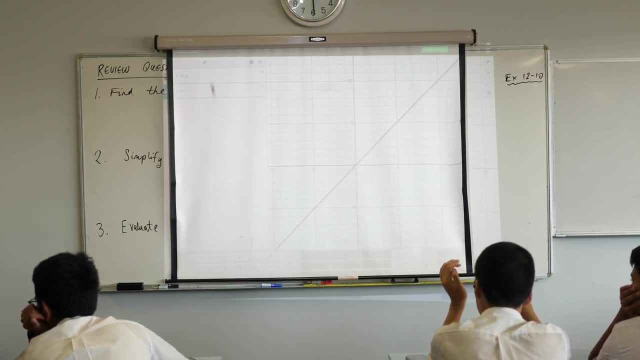 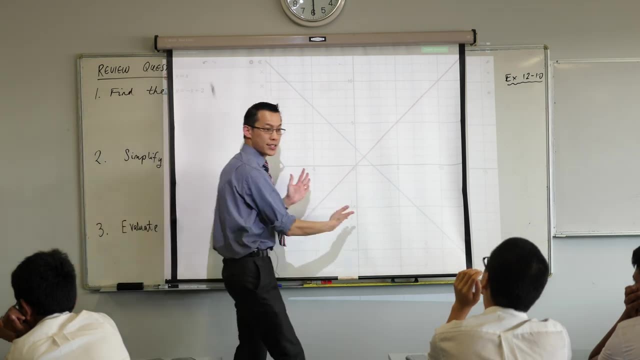 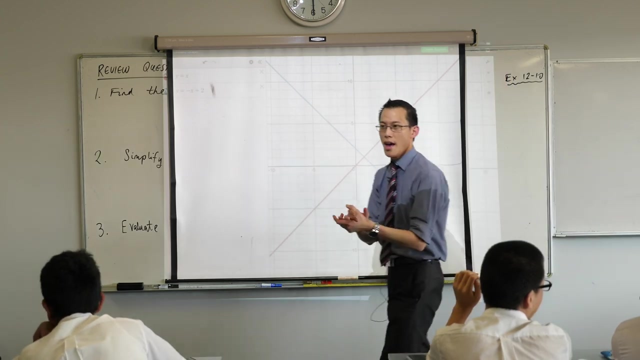 y equals what is it? y equals what? Yeah, negative x plus 2.. Okay, now can I get a show of hands? who has this on this screen right now? Who's up to speed? Yeah, hands up, hands up, hands up, about half the class. Okay, thank you, hands down, All right now. before we inspect this, I just want to pause on. 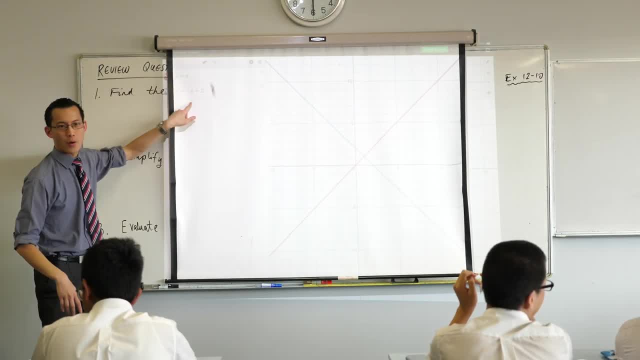 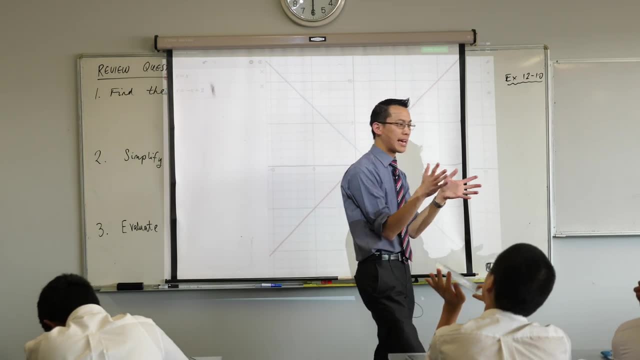 some of the language that we learned before. Okay, so have a look at our equations that you can see here: y equals x, y equals negative, x plus 2.. There were two words that we looked at last lesson. that was super important. we're going to use them. 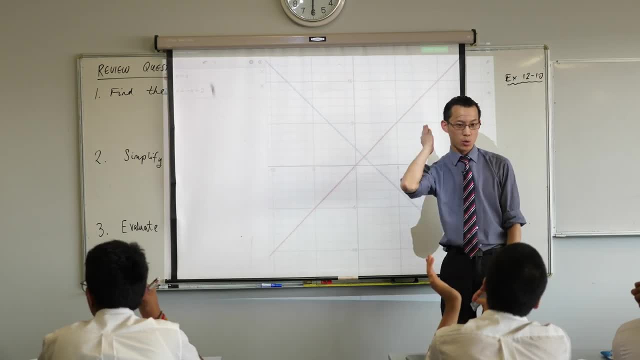 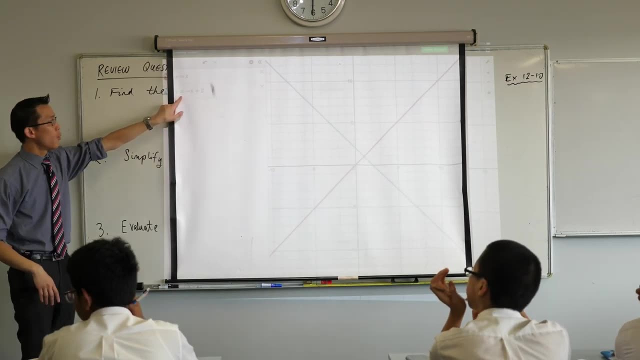 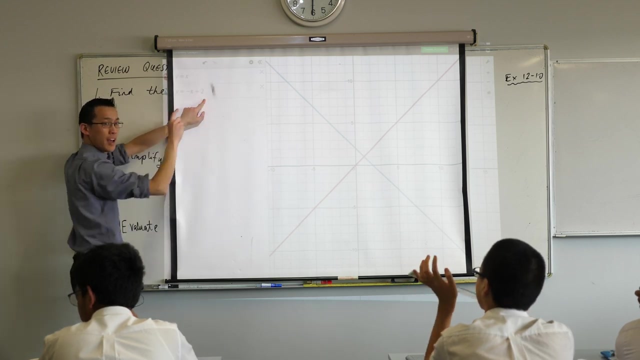 again and again. They both started with the letter c. One is called the coefficient and one is called the constant. Very good, can you help me work out? let's look at this second one. What's the constant in this second equation? The constant is it's two. it's this number over here, right, a bit trickier. 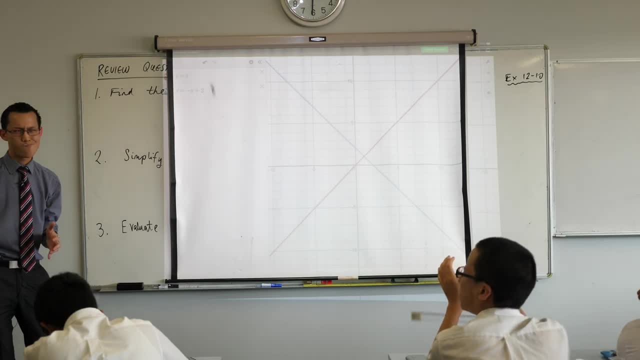 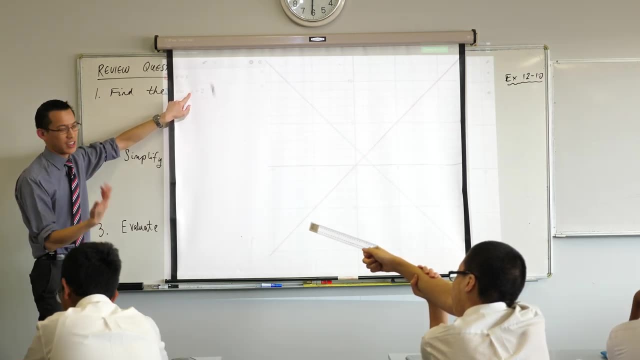 what's the coefficient in that same equation? That's tricky. the coefficient's the number that's in this case is a negative one. we don't write the one because it kind of doesn't change anything. it's the same size. Okay, what about the first equation? What's the constant in the first? 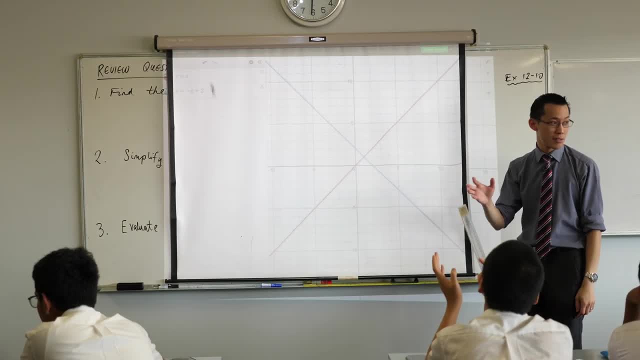 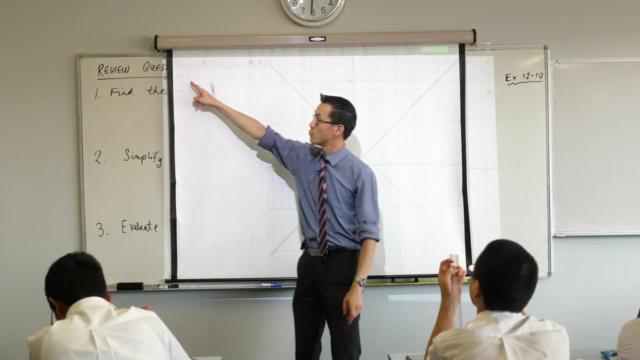 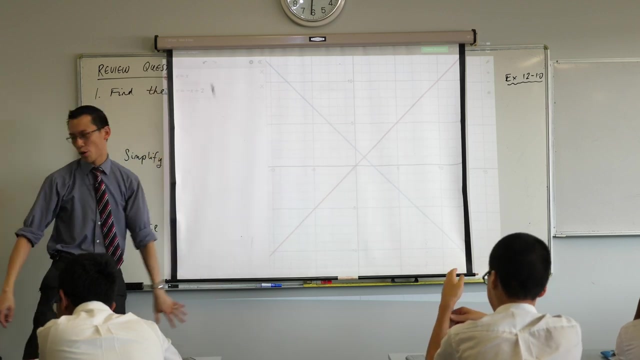 equation. It's sort of hiding right, it's plus zero. that's why we don't write. it doesn't change anything. What's the coefficient in the first one? It's just one. it's just hiding there one times. x is just x. that's why it's not written. Okay, now, this is what you've got. have a look in closer. 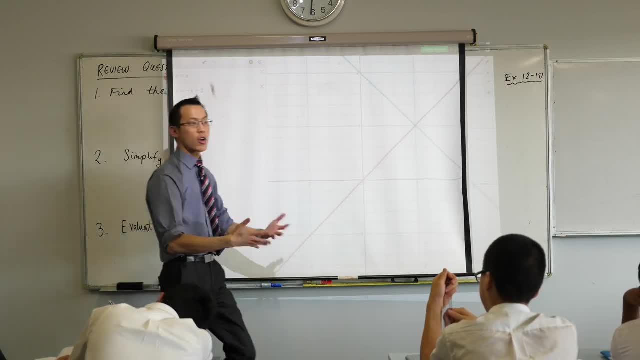 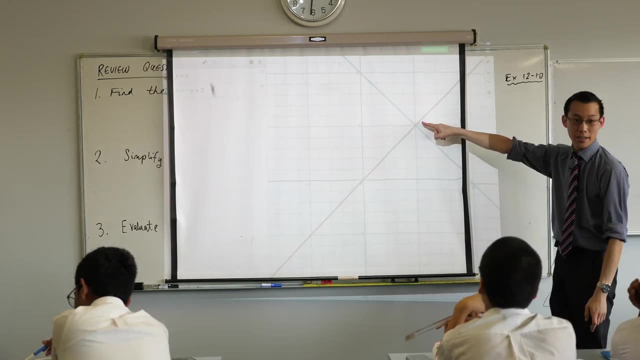 and what we want is that point where they, as William said, cross paths. that's the point of intersection. so have a look. can you guys read off for me what's the x coordinate of this point? It's one you can read there- and what's the y coordinate? Coincidentally, it's the same, so go ahead in. 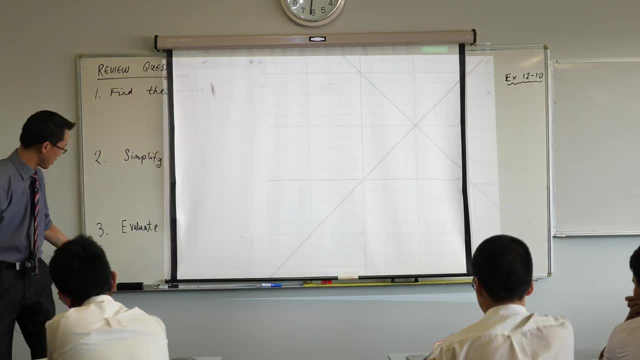 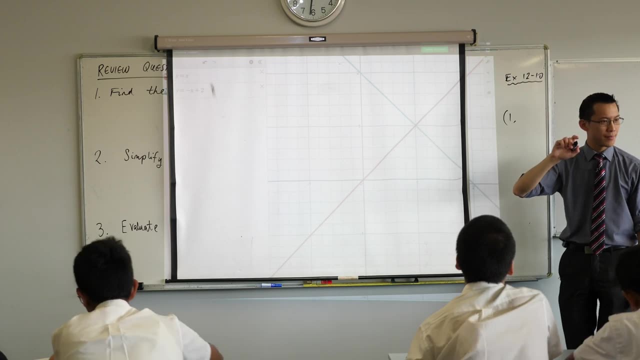 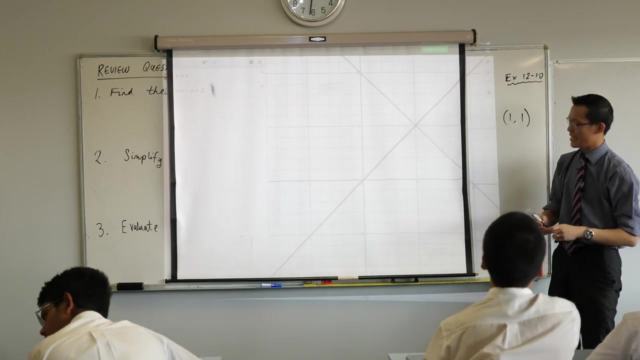 question 1a: we write the coordinates, don't forget, in a very particular way to indicate that it's a point. right, those two values that you just gave me: the x coordinate is the first number and the y with a comma, and we've got those two parentheses around to indicate this is a point. okay, now I'm. 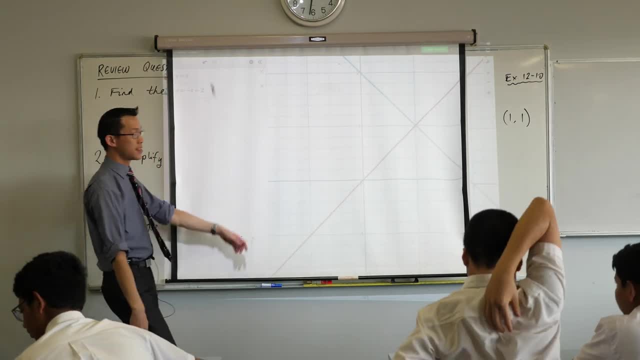 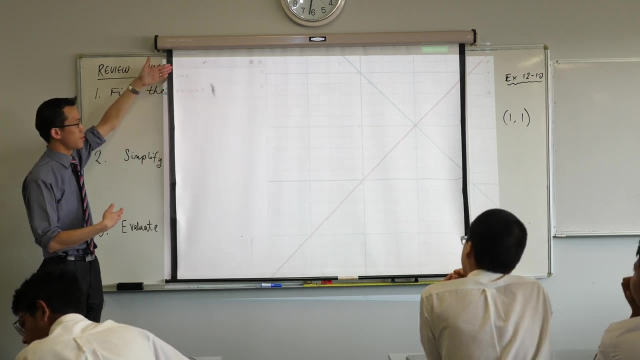 going to give you a second to have a look at 1b. there's two different equations there and I invite you, rather than having like a million equations here, which is going to be very confusing, just change these two equations, the ones that are there at the moment. they're probably red and blue, like. 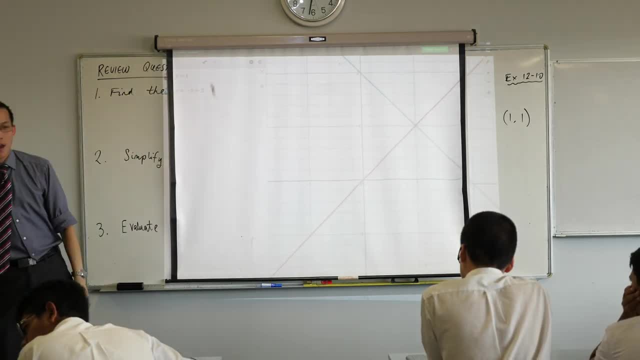 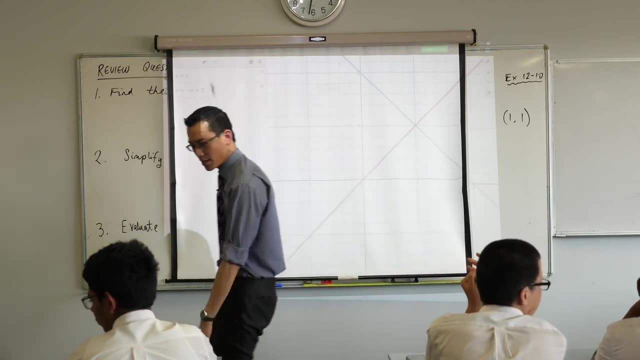 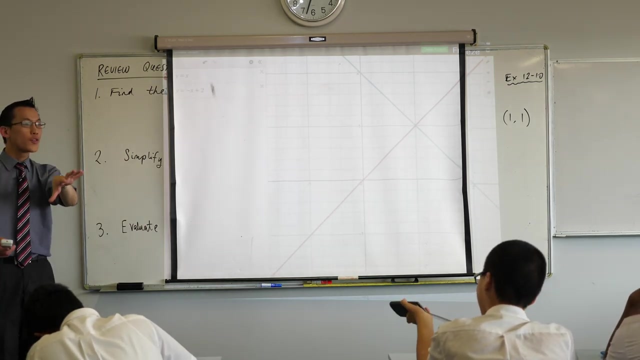 mine. go ahead and adjust those two so that they match the question, or rather the equations in part b. can you do that and then see if you can find the point of intersection? okay, so have a look up. has what have you? what you've got on your screen, does it match this? 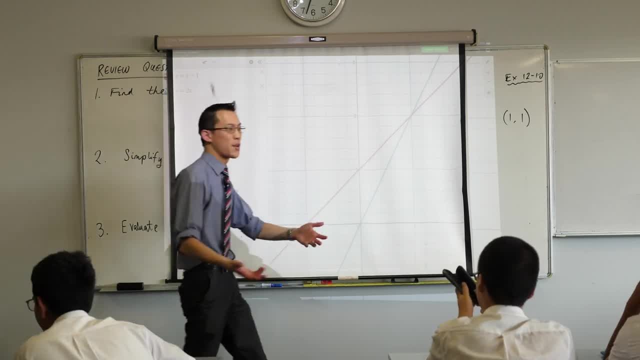 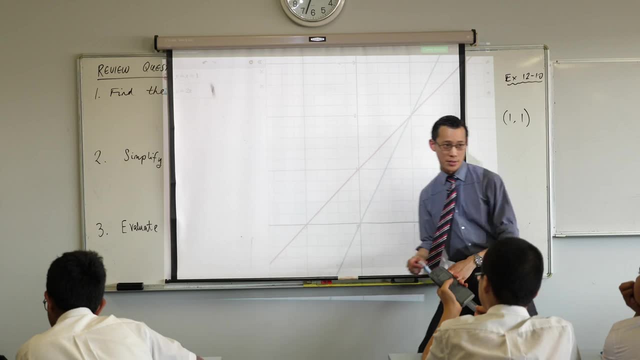 is that what looks like? maybe you're red and your blue is swapped over. it doesn't really matter which one's which. okay. so this time again we've got a point of intersection. what is the point of intersection? what are its coordinates? 1 comma 2: very good again. the first value is the x, which is: 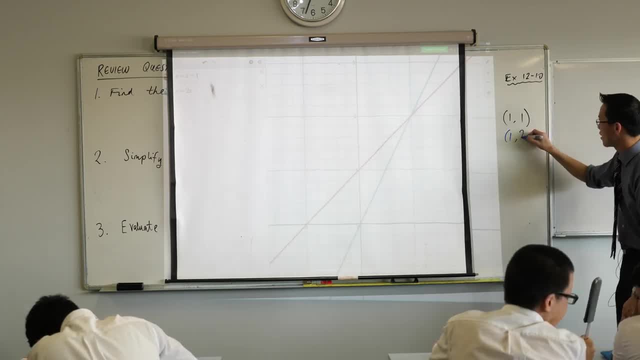 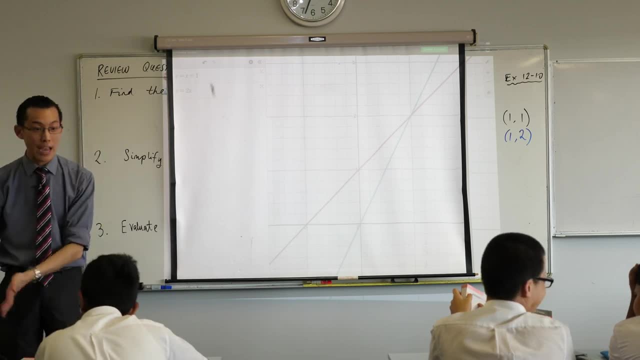 horizontal. there's the one which we can see up there, and your second value is the 2. okay, now here's what I'd like you to do. I'd like you to do is you're going to go to the next one and you're going to finish question one again, use the technology every time, but what I want you to 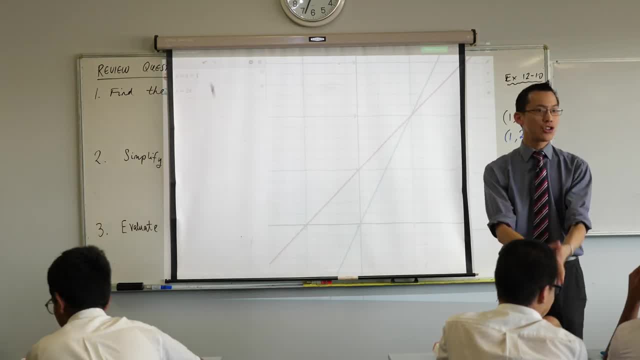 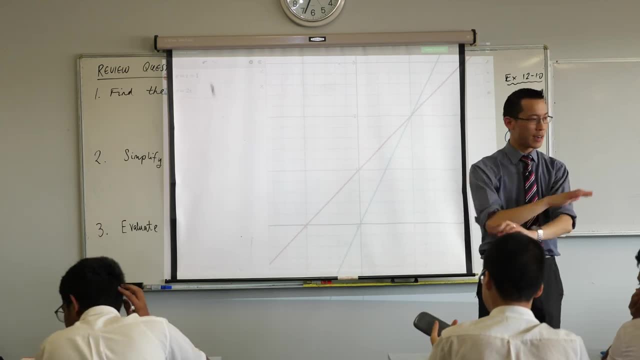 lastly do is. this is why I asked you to have rulers. I want you to choose one of the questions a, b, c, d, e or f- I don't mind which one you choose- and I want you to physically draw that one in your book. you don't have to draw all six. you can use technology for all six, but I do want you to. 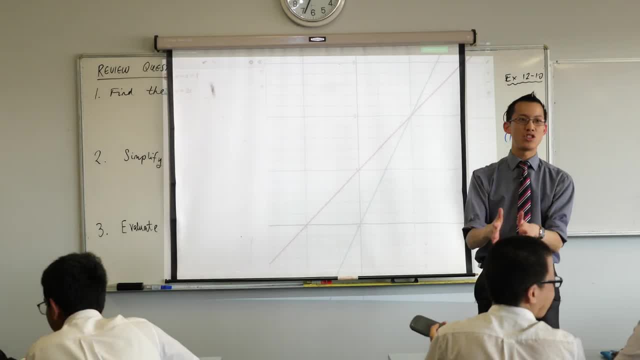 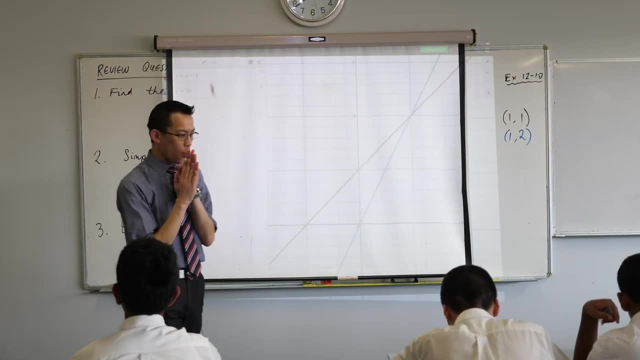 physically draw at least one of them in question one into your book. show the two lines, show the point of intersection. I'll let you choose which one you want. okay, when we have a look at questions two and three, I don't want you to just march through. I want you. 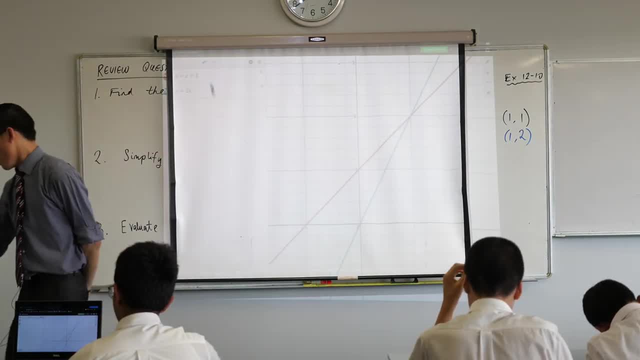 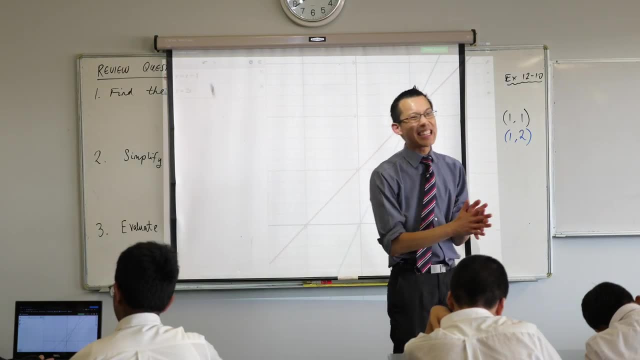 to think about it in a particular way. so look at it with me. it says question two: what's the point of intersection? and then they provide you with two lines, just like we've been looking at before. in some ways that's exactly like question one, no big deal. so you can go ahead with that in a second. 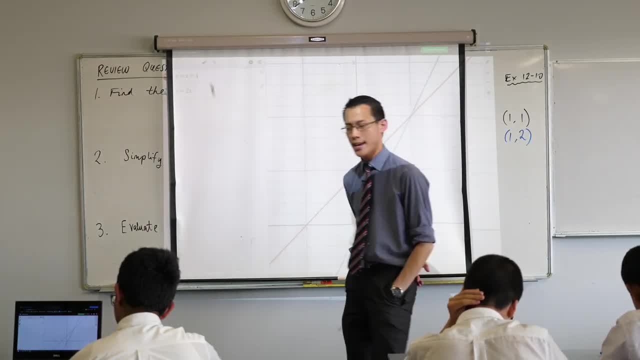 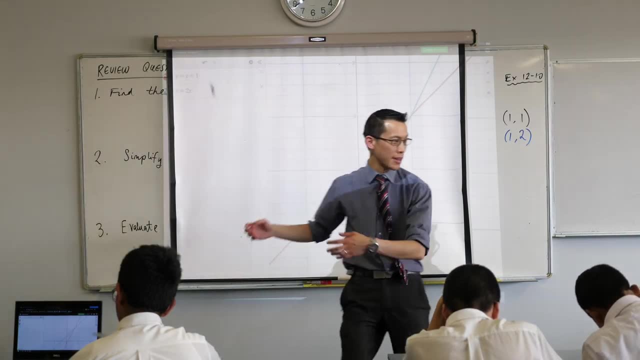 question three, though it's a bit differently different. can you have a look at it with me? it says: solve each equation graphically. now, when we say graphic, and what we mean is like this: with the aid of graphics, by graphing them and you can see what the solutions are. and 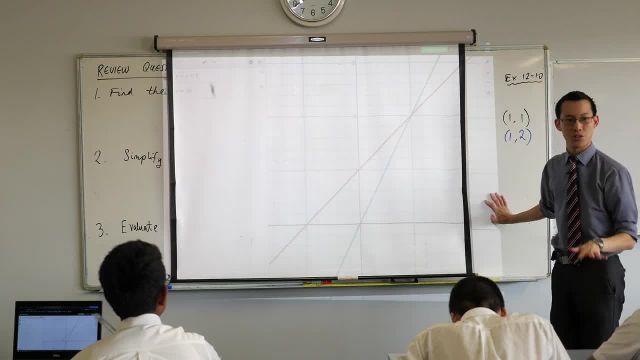 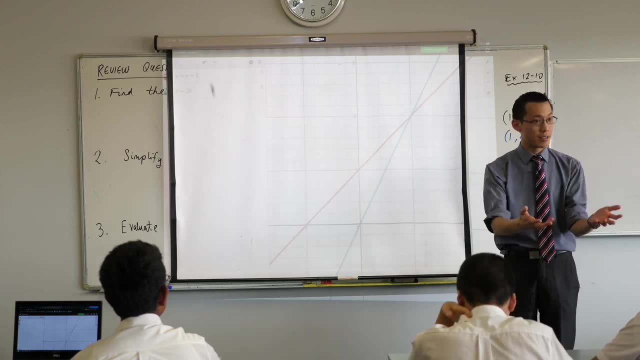 then read what it is okay. the weird thing is, if you have a look closely at question three, the parts look very different from what we've got. there's no y equals this. there's no y equals that. you've just got x's. here's what they mean. open your lids up again and instead of the two equations you had, 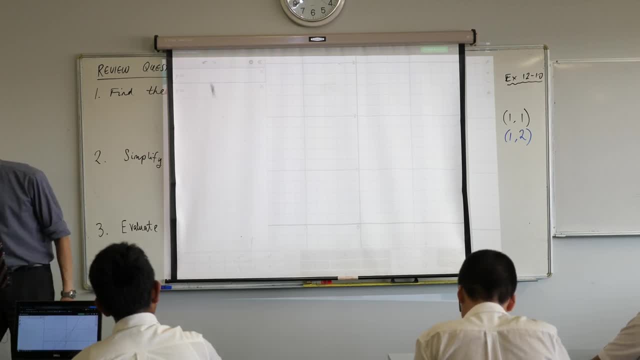 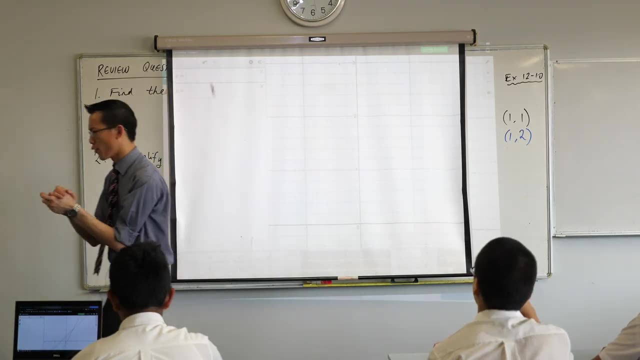 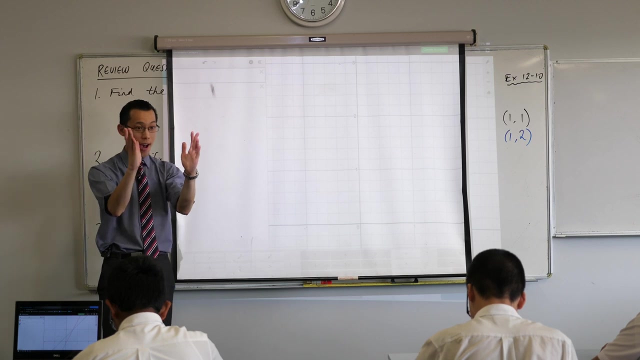 before, replace them with the left hand side and the right hand side of those two equations or the equation you can see in question three. so for example, in fact i can even get rid of the y equals in the top line. i'm just going to write the left hand side of the equation in 3a which says 2x is: 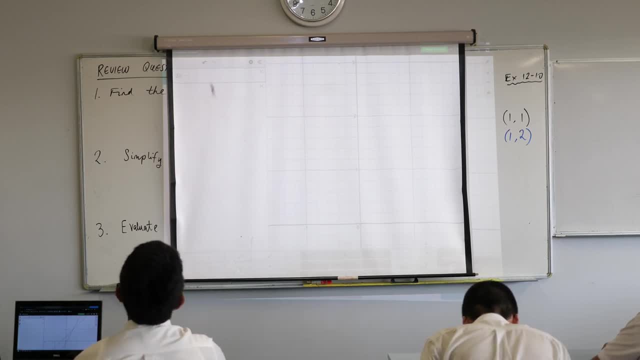 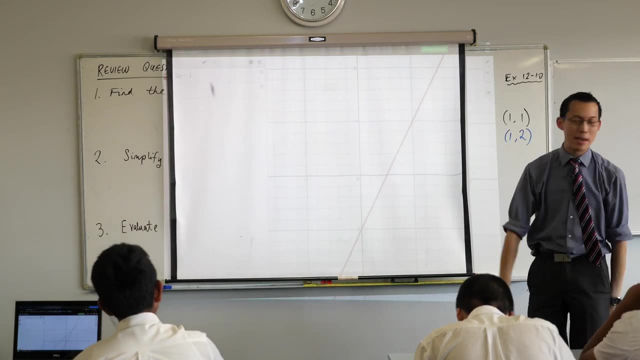 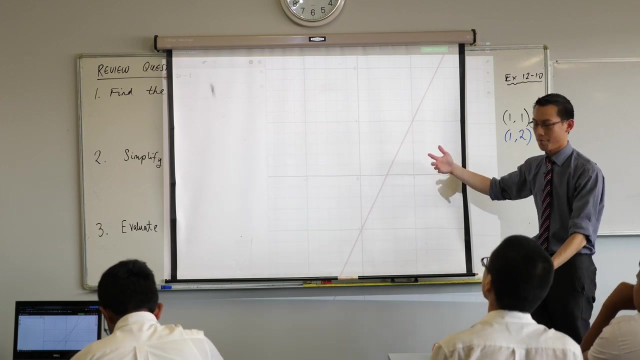 it 2x minus 1.. okay, now, when you put in 2x minus 1 by itself, Desmos is guessing that you mean y equals this, and that's why you can see a graph. right, this is the two x minus one part of the graph. then we can put on the line beneath the right hand side of the equation: it's. 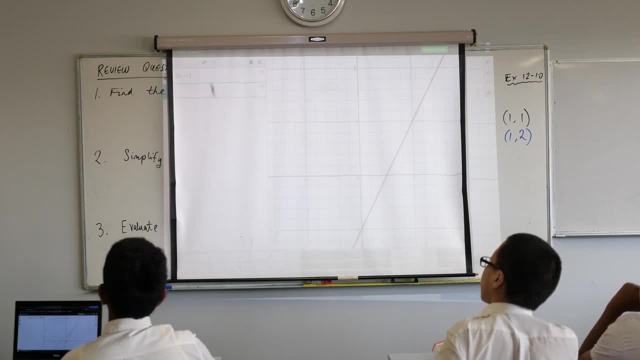 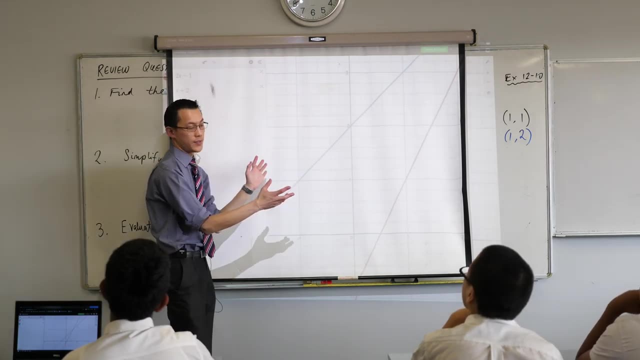 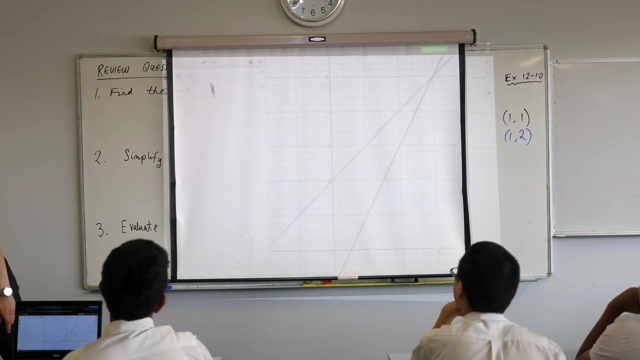 x plus two. x plus two. now you may need to, as just like I do. you may need to move the part of your graph that is visible so you can see the point of intersection. you might need to zoom out as well. eventually you'll see. can you help me, whoops? can you help me read off what the solution is for this? 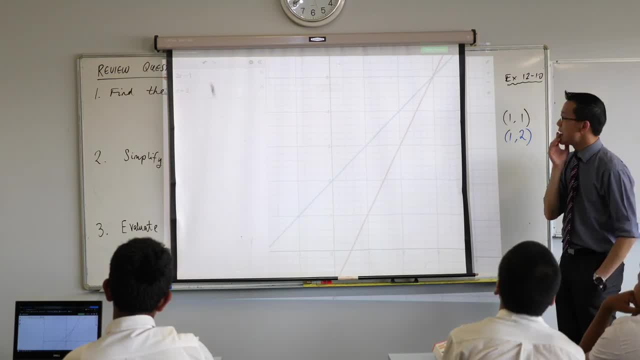 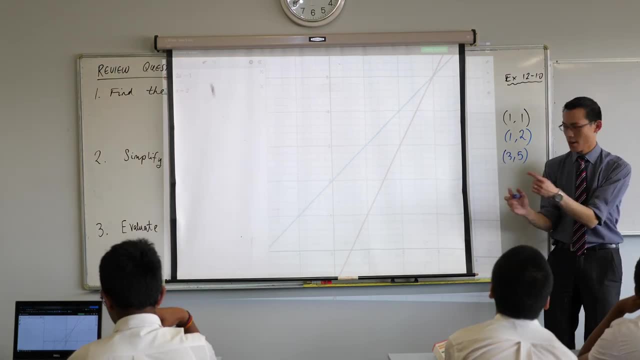 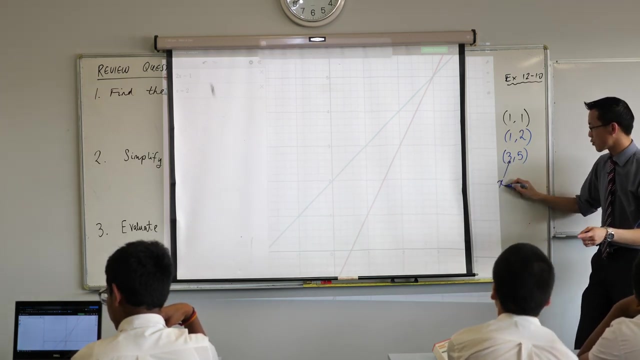 what's the, what's the coordinates? where's the point of intersection? three, three comma five, right, so I can write that down: three comma five. but I want to ask you guys which number is which? which one's the x and which one's the y? this is the x, right? this is the y. now look back at the original question, do you notice? 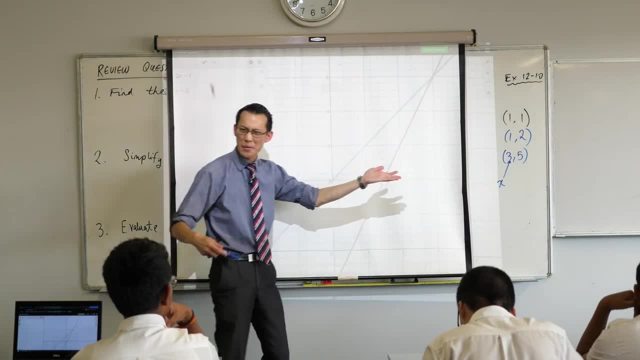 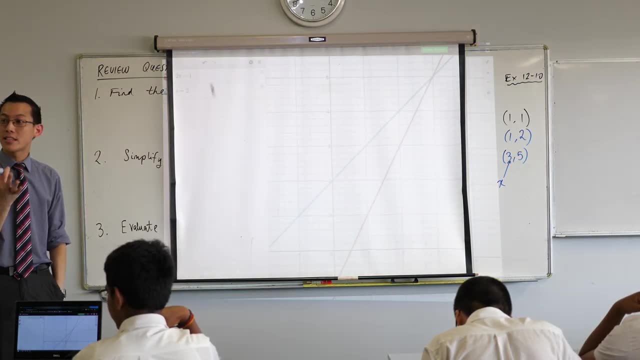 it doesn't have any y's in. that's what I was highlighting. so which of these numbers do I really care about? look at the question. it's a question that's all about what is the answer. so let's say what is part of the vertical? it's all about x, right? so therefore I 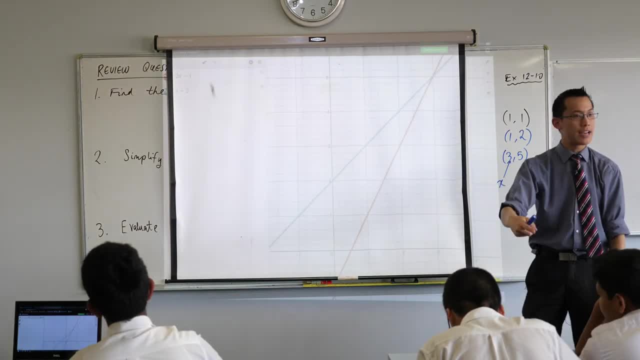 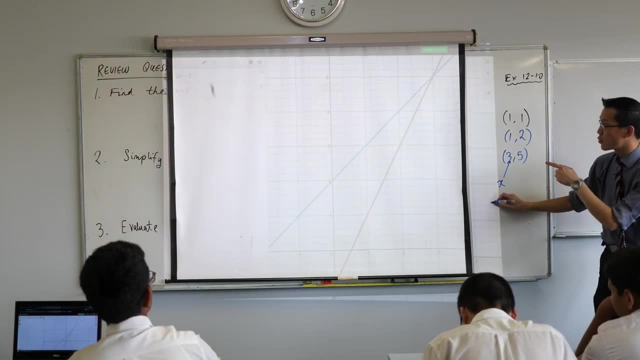 use this and I say: the part that I'm focusing on is the x. now, question four underneath asks you to confirm this just by doing it with algebra, which we can do right now. pick up your pen. these equation. this equation was two x, what was it? minus one equals four x plus two. all right, 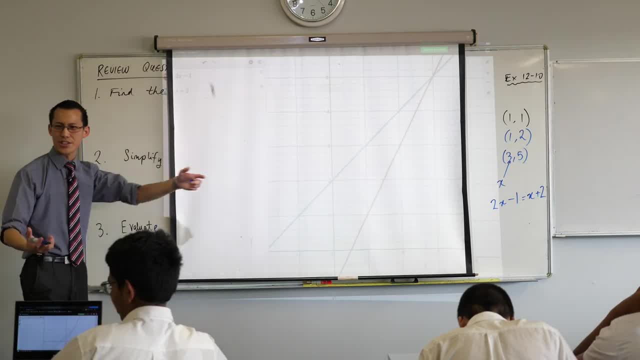 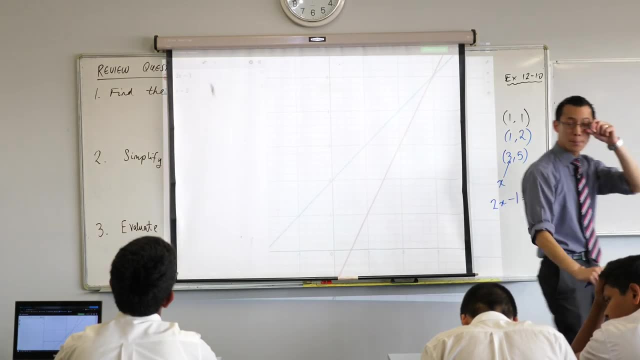 alright, ok now if we didn't have a graph, we could just solve this as an equation. we could probably take two steps. what could be something we do? bright burden, apply again, marked zero, this simpler. and they, what do you say? we switch the minus one and the X. so I'm 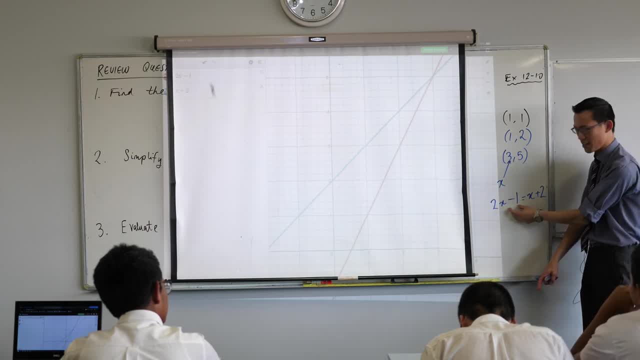 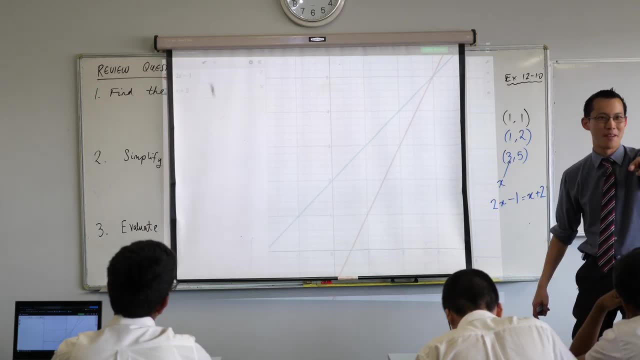 guessing. what you mean is: how do we switch? by the way, like I don't want this minus one to be here, what do I do to both sides to get rid of it? hmm, ah, that's interesting. I actually could multiply by minus one, but it would just. 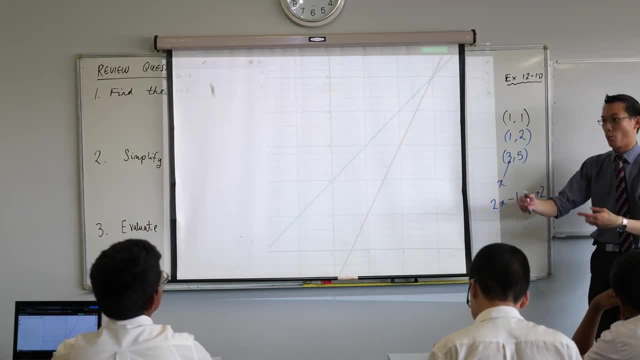 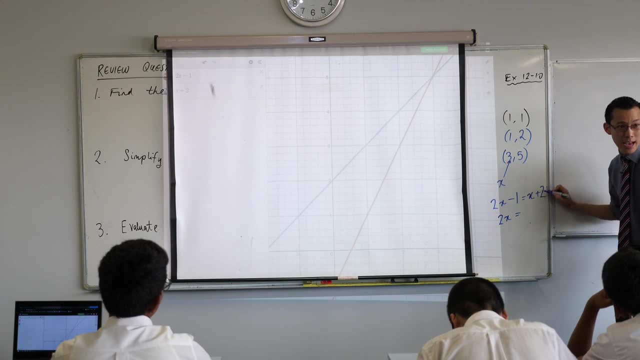 turn it into a plus one, so it's sort of still be there. the rest of you said we could add one that'll get rid of this here, which would make this not plus two. when you add one to both sides it'll become plus three, and then I need one. 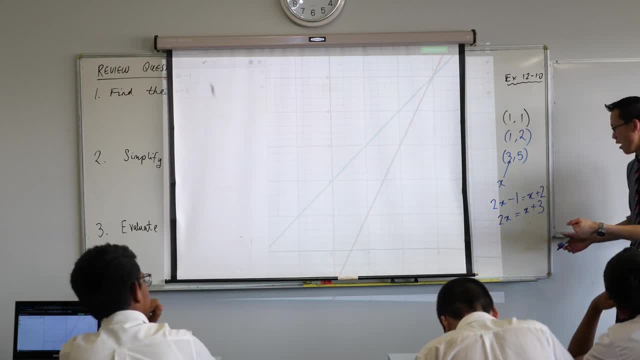 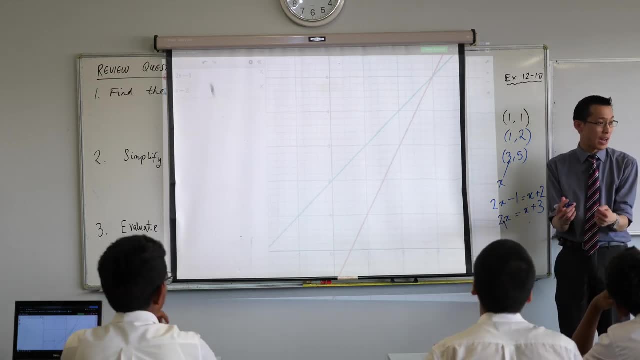 more step. what was the other thing I need to do? an ish, ah, minus two. now I have it to here, but actually this is kind of a different operation hiding there, right? what's the operation that's hiding its multiplication? what's the thing I used to undo that division, right? 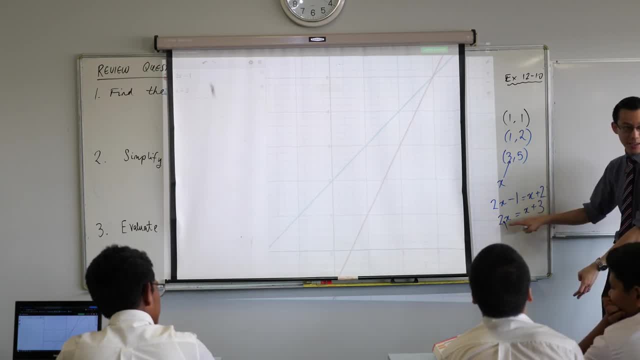 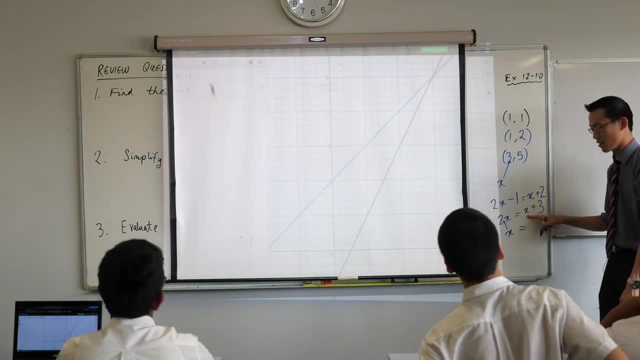 so I should divide both. oh, if I divide both sides by two, I would get more X's over here. I think we could subtract X right. so I'm going to subtract X from here, and then I'm going to subtract X from here. what do we get? which is what we.